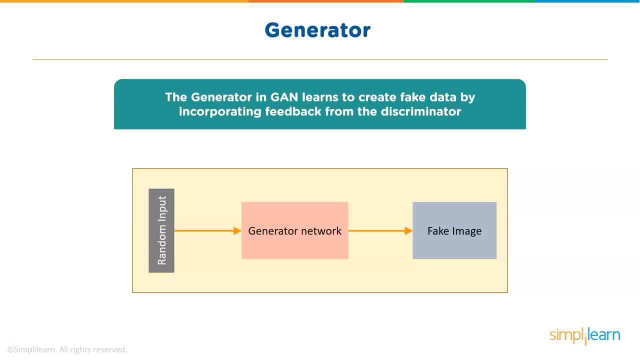 examples for the discriminator. It takes a fixed length random vector carrying noise as input and generates a simulator. It can also generate random variables. When the data is generated, it had a run value of half the value. The data input used in GANs is 0.016.. 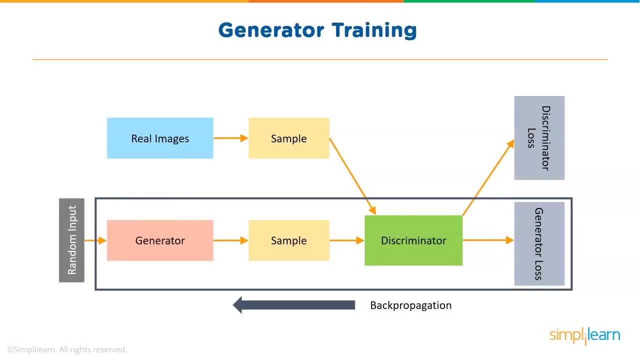 Now, the main aim of the generator is to make the discriminator classify its output as real. The portion of the GAN that trains the generator includes a noisy input vector, the generator network, which transforms the random input into a data instance, a discriminator network. 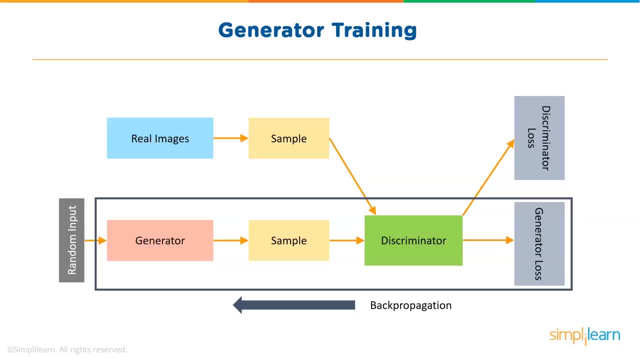 which classifies the generated data, and a generator loss, which penalizes the generator for failing to dolt the discriminator. The backpropagation method is used to adjust each weight in the right direction by calculating the weight's impact on the output. The backpropagation method is used to obtain gradients, and these gradients can help change. 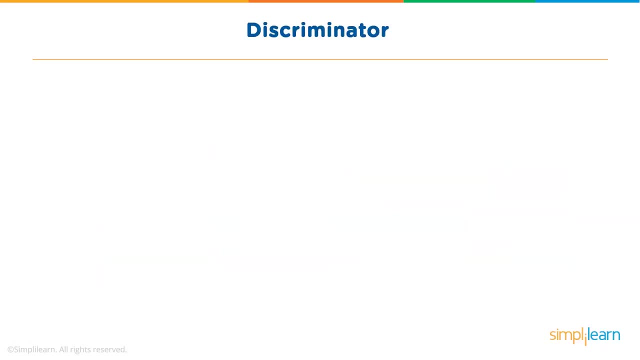 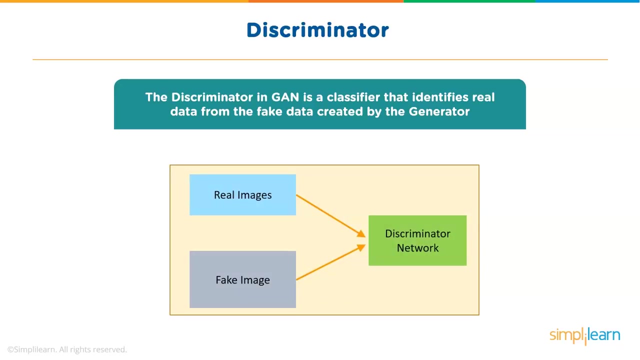 the generator weights. Now let us understand in brief what a discriminator is. A discriminator is a neural network model that identifies real data from the fake data generated by the generator. The discriminator's training data comes from two sources: The real data instances, such as real picture and real data. 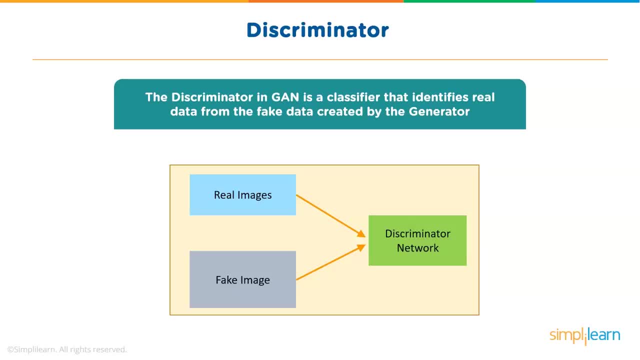 So birds, humans, currency notes, etc. are used by the discriminator as positive samples during the training. The fake data instances created by the generator are used as negative examples during the training process. While training the discriminator, it connects with two loss functions. 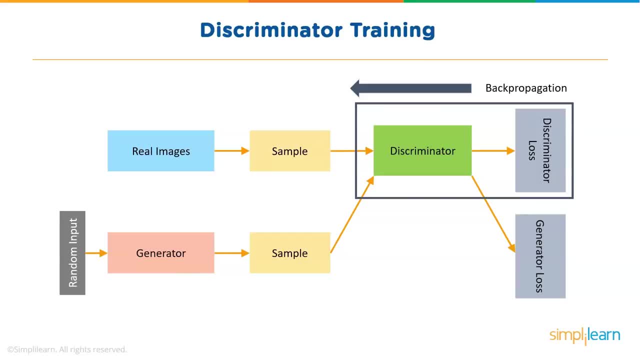 During discriminator training, the discriminator ignores the generator loss and just uses the discriminator loss In the process of training the discriminator. the discriminator classifies both real data and fake data from the generator. The discriminator loss penalizes the discriminator for misclassifying a real data instance, as 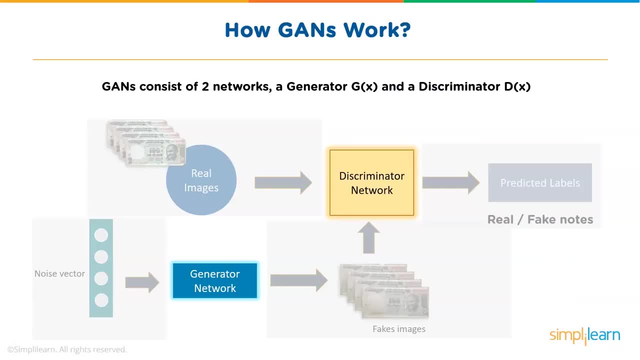 fake or a fake data instance as real. Now, moving ahead, let's understand how GANs work. GANs consist of two networks: a generator, which is represented as G, and a discriminator, which is represented as D. They both play an adversarial game, where the generator tries to fool the discriminator. 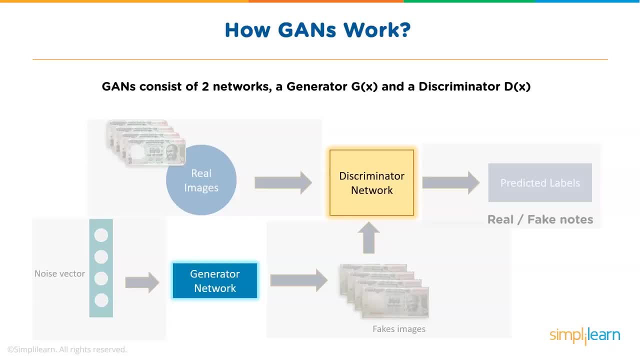 by generating data similar to those in the training set. The discriminator tries not to be fooled. The discriminator tries not to be fooled by identifying fake data from the real data. They both work simultaneously to learn and train complex data like audio, video or image. 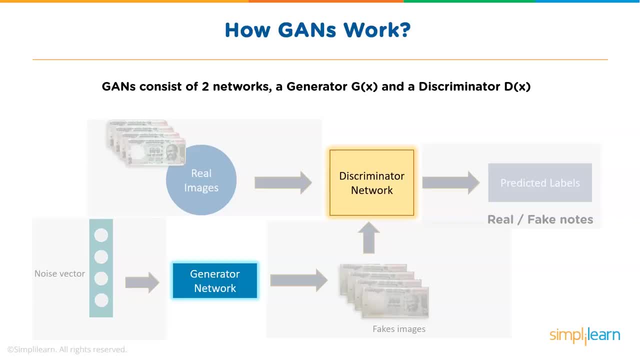 files. Now you are aware that GANs consist of two networks: a generator G and a discriminator D. Now the generator network takes a sample and generates a fake sample of data. The generator is trained to increase the probability of the discriminator network to make mistakes. 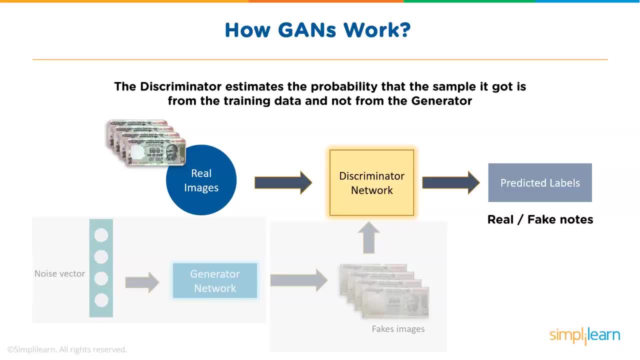 On the other hand, the discriminator network decides whether the data is generated or taken from the real sample using a binary classification problem, with the help of a sigmoid function that gives the output in the range 0 and 1.. Here is an example of a generative adversarial network trying to identify if the 100 rupee 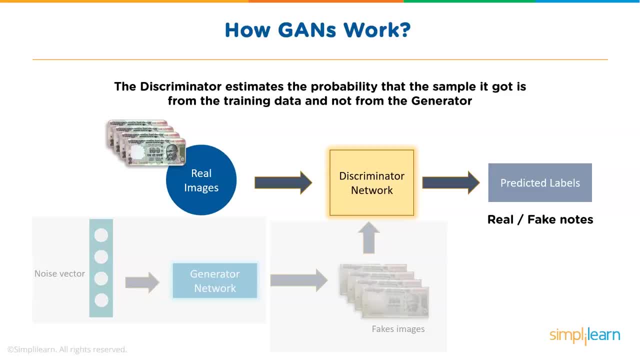 notes are real or fake. First a noise vector or the input vector is fed to the generator network. The generator creates fake 100 rupee notes. The real images of 100 rupee notes stored in a database are parsed to the discriminator along with the fake notes. 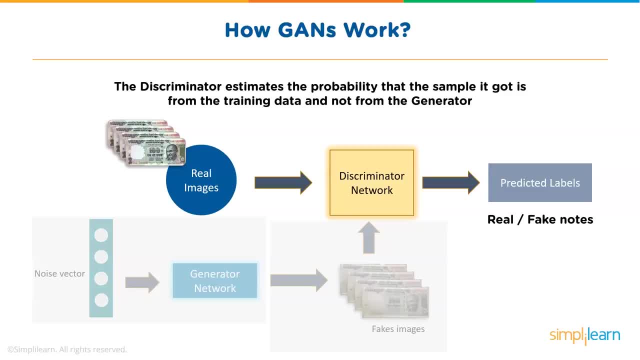 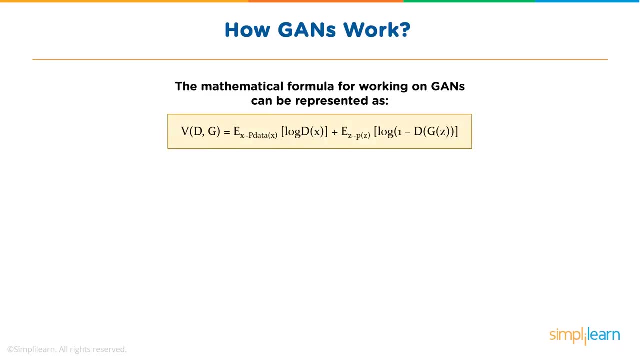 The discriminator then identifies the notes and classifies them as real or fake. We train the model, calculate the loss function at the end of the discriminator network and back propagate the loss into both discriminator and generator. Now the mathematical equation of training again can be represented as you can see here. 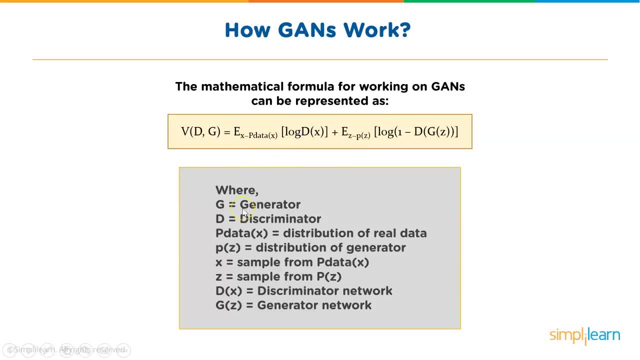 Now this is the equation and these are the parameters Here. G represents generator, D represents the discriminator. Now, p data of x is the probability distribution of real data. P of z is the distribution of generator. X is the sample of probability data of x. 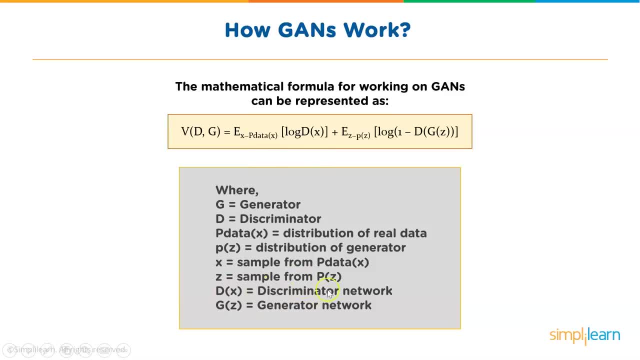 Z is the sample size from p of z. D of x is the discriminator network and G of z is the generator network. Now the discriminator focuses to maximize the objective function, such that D of x is close to 1 and Z of z is close to 0.. 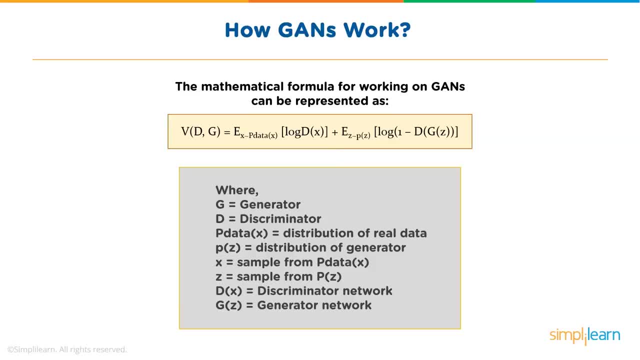 It simply means that the discriminator should identify all the images from the training set as real. All the generated images are fake. that is 0.. The generator wants to minimize the objective function such that D of z of z is 1.. This means that the generator tries to generate images that are classified as real, that is. 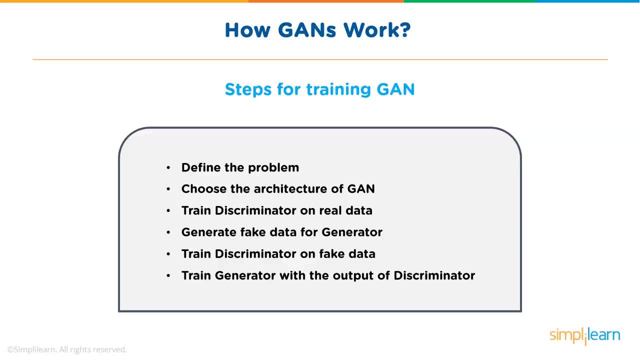 1 by the discriminator network. Next let's see the steps for training a neural network. So we have to first define the problem and collect the data. Then we'll choose the architecture of GAN. Now, depending on your problem, choose how you're going to use it. 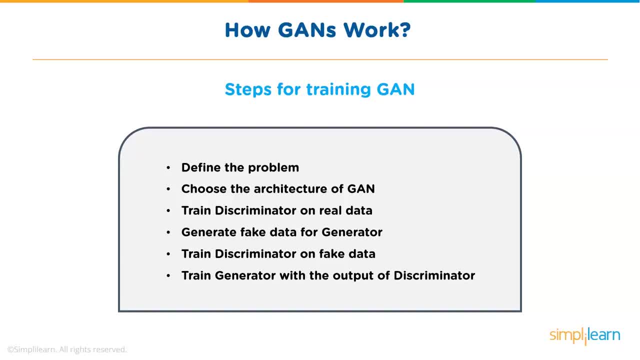 First we need to know what GAN should look like. Then we need to train the discriminator on real data. That will help us predict them as real for n number of times. Next, you need to generate fake inputs for the generator. After that, you need to train the discriminator on fake data to predict the generator data. 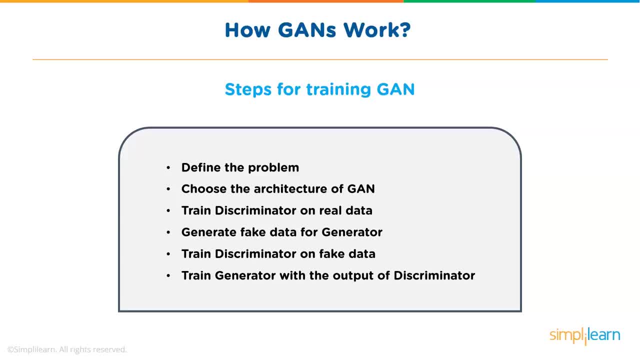 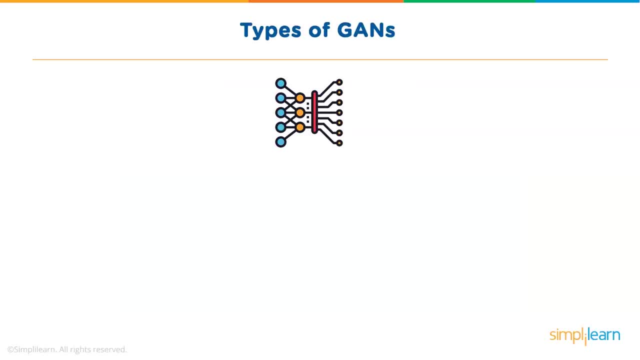 as fake. Finally, train the generator on the output of discriminator With the discriminator predictions available. train the generator to fool the discriminator. Let us now look at the different types of GANs. So first we have Vanilla GANs. Now Vanilla GANs have min-max optimization formula that we saw earlier, where the discriminator 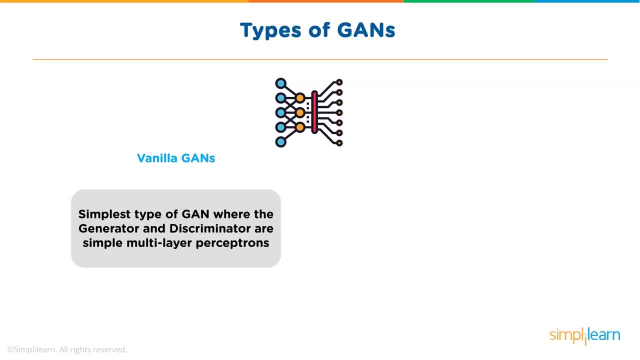 is a binary classifier and is using sigmoid cross entropy loss during optimization. In Vanilla GANs, the generator and the discriminator are simple multi-layer perceptrons. The algorithm tries to optimize the mathematical equation using Stochastic Gradient Descent. Up next we have Deep Convolutional GANs, or DC GANs. 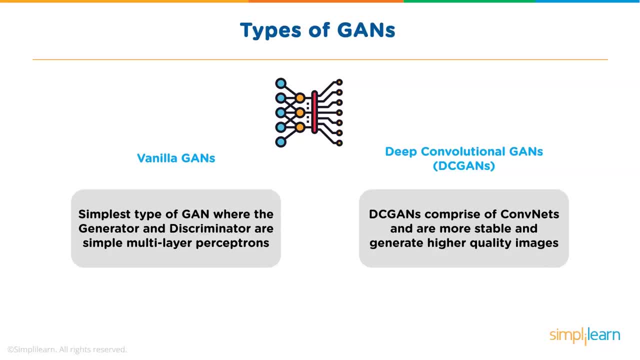 Now DC GANs support convolutional neural networks instead of vanilla neural networks at both discriminator and generator. They are more stable and generate higher quality images. The generator is a set of convolutional layers with fractional strided convolutions or transposed convolutions, so it unsamples the input image at every convolutional layer. 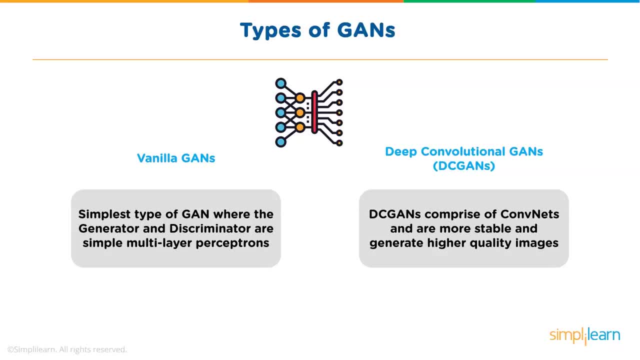 The discriminator is a set of convolutional layers with strided convolutions, so it downsamples the input image at every convolutional layer Moving ahead. The third type we have is Conditional GANs or C GANs. Vanilla GANs can be extended into conditional models by using an extra label information. 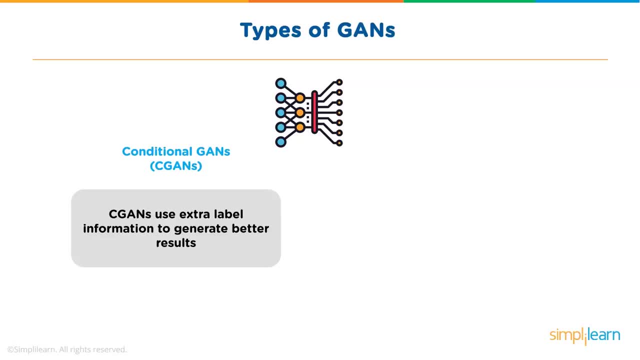 to generate better results. In C GAN, an additional parameter called y is added to the generator for generating the corresponding data. Labels are fed as input to the discriminator to help distinguish the real data from fake data generated. Finally, we have Super Resolution GANs. 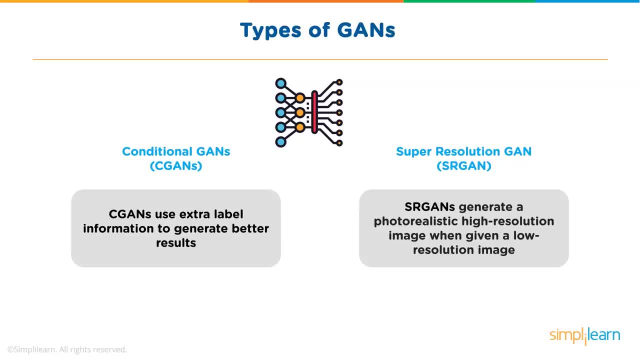 Now SR GANs use deep neural networks along with adversarial neural networks. Super Resolution GANs generate photorealistic high-resolution images Once the resolution startsivoing is positive. the GANs are then represented as 2D physics that need a super practical application.